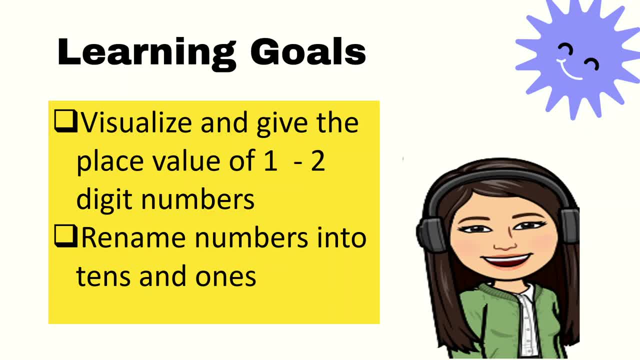 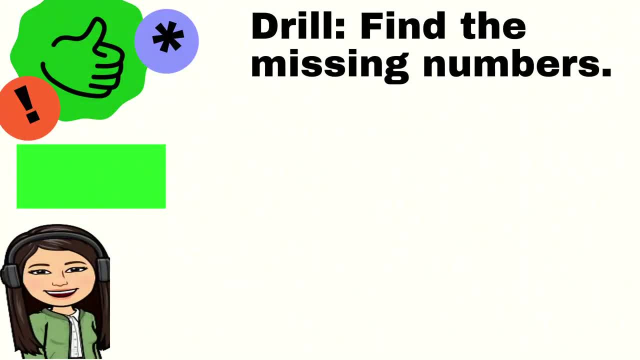 and to rename numbers into tens and ones. But before that, let us recall our lesson on counting numbers up to 50.. Find the missing numbers, Okay. so find the missing numbers, Ready Go? Okay, let's check. So if we count starting from 39,, next is 40. What's next after 40?? 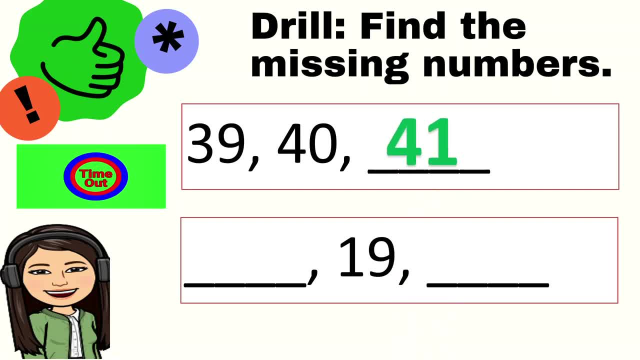 Yes, it's 41.. What about the number before 19?? Yes, it's 18.. And after 19? It's 20.. Very good, Okay. next, What about this? Find the missing numbers Ready Go. 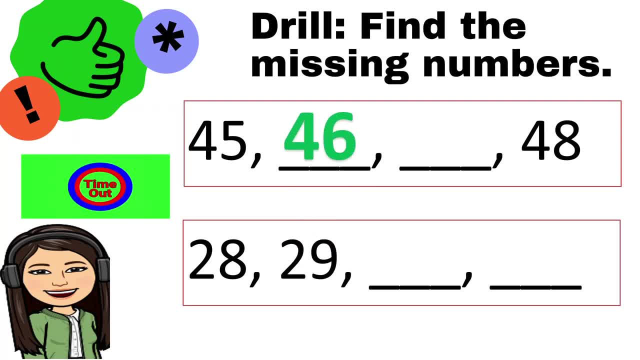 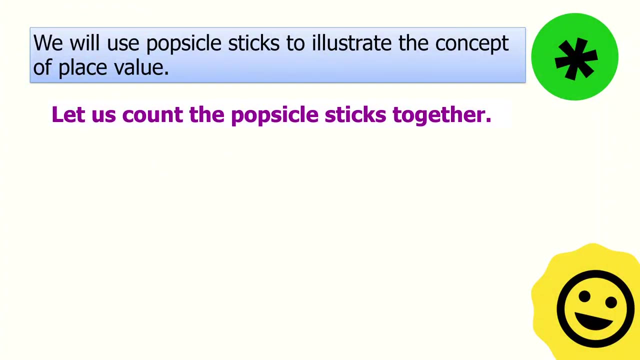 Alright, let's check. Okay, after 45,, 46, and then 47 and 48. Very good. Next, 28,, 29,, 30, and then 31.. Yay, Very good. Okay, now We will use popsicle sticks to illustrate the concept of place value. 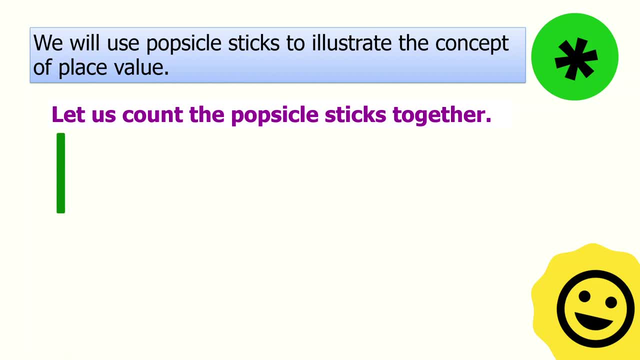 Let us count the popsicle sticks together: 1,, 2,, 3,, 4,, 5,, 6,, 7,, 8,, 9,, 10,, 11,, 12,, 13,, 14,, 15,, 16,, 17,, 18,, 19,, 20,, 21,, 22,, 23,, 24,, 5,, 6,, 7,, 8,, 9,, 10,, 11,, 12,, 13,, 14,, 15,, 16,, 17,, 18,, 19,, 20,, 21,, 22,, 23,, 24,, 5,, 6,, 7,, 7,, 8,, 9,, 10,, 11,, 12,, 13,, 14,, 14,, 15,, 16,, 17,, 18,, 19,, 20,, 21,, 22,, 23,, 24,, 5,, 6,, 7,, 7,, 8,, 9,, 10,, 11,, 12,, 13,, 14, 14,, 15,, 16,, 17,, 18,, 19,, 20,, 21,, 22,, 23,, 24,, 5,, 6,, 7,, 7,, 8,, 9,, 10,, 11,, 12,, 23,, 24,, 5,, 6,, 7,, 7,, 8,, 9,, 10,, 12,, 23,, 24,, 5, 6. 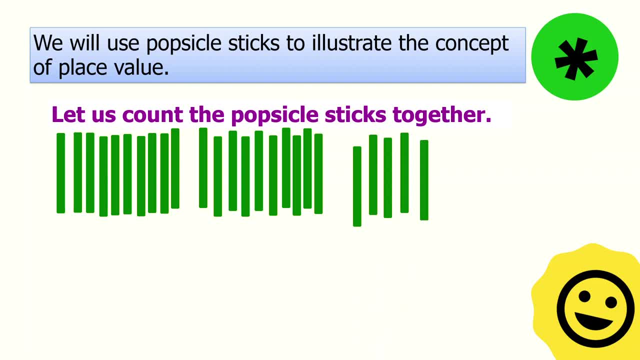 24, 25, all right, so let us group these sticks into 10, so we have this first group of 10 and another group of 10, and so we have the others. there are five popsicle sticks left, not by. you can't group it by 10 because it's not enough, right? we cannot make one group of 10. so how many groups? 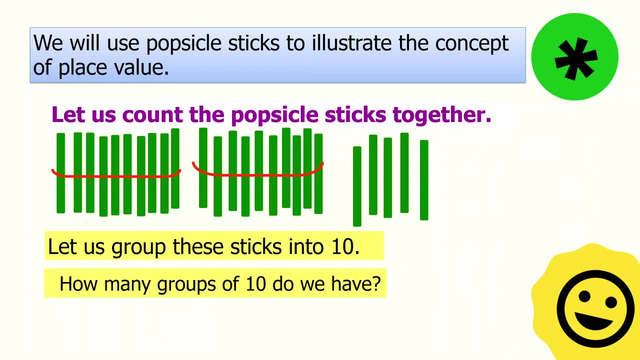 of 10? do we do we have there? right, we have two, okay, so we have two groups of tens, okay. and then, how many ones are there? can you count? yes, we have five ones, all right. so what is the number that we form? it's 25, right, it's 25.. now, what is the place value of two? 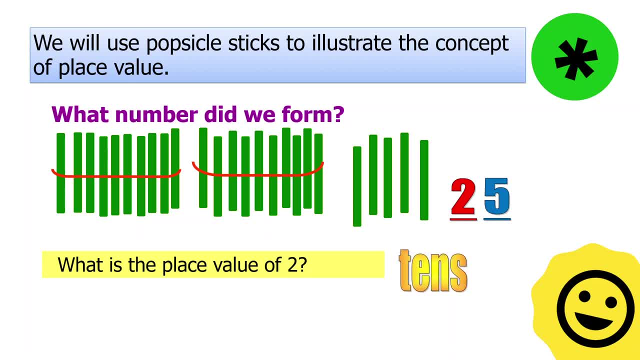 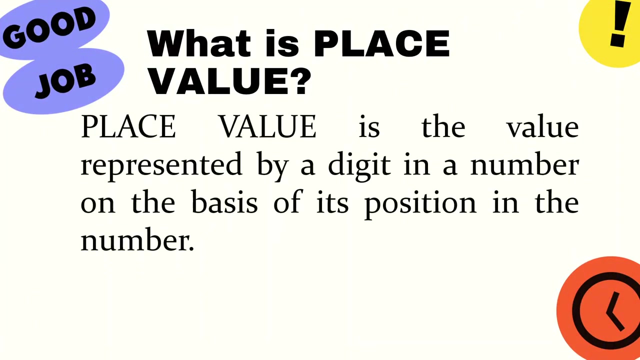 tens. yes, it's tens, because we have two groups of tens: two tens, the place value of the tens. we do have 25 and then five numbers. Eduardo Unruly members didn't have a chance, so they didn't have positive numbers on the top, so the one that you asked for would be positive years, whether you want one or two. 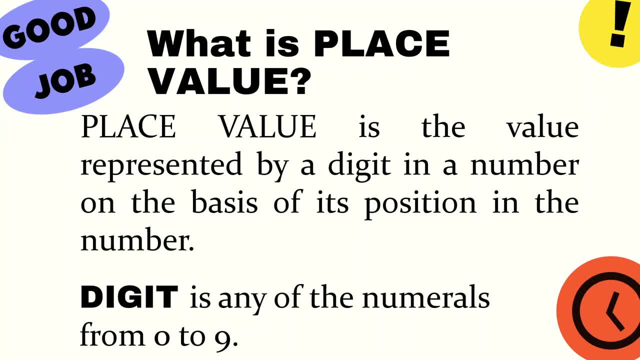 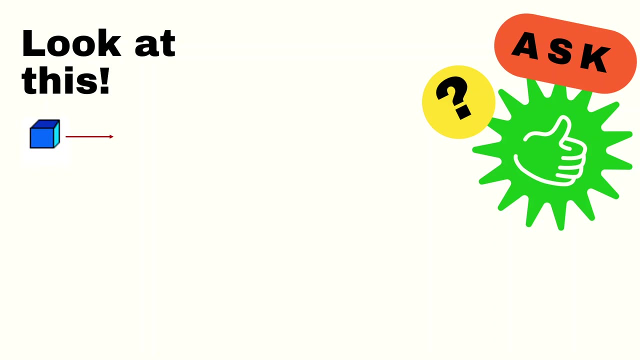 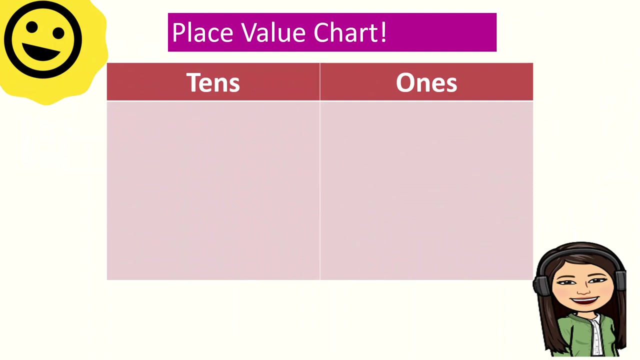 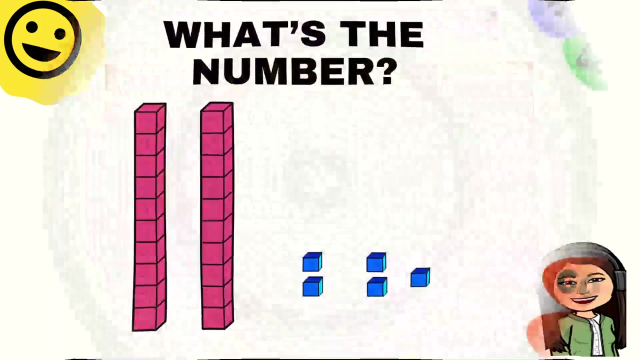 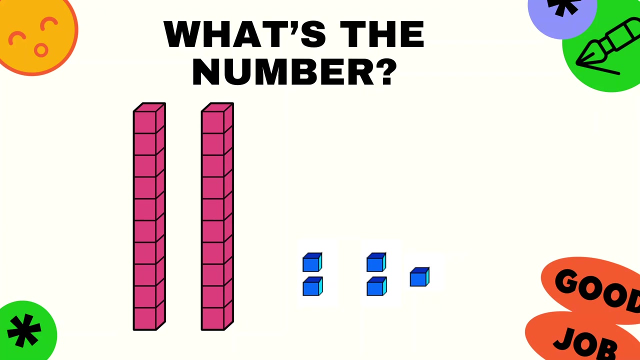 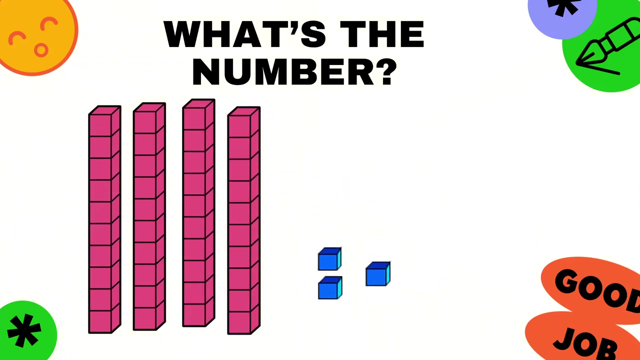 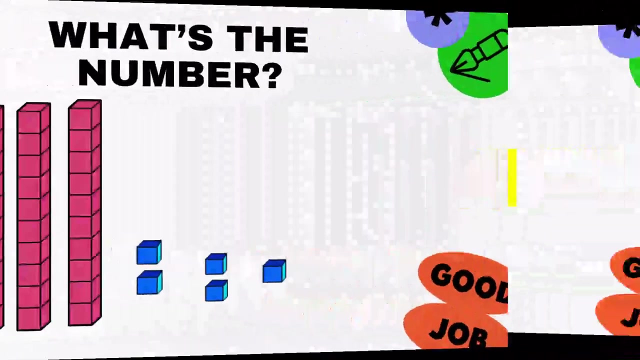 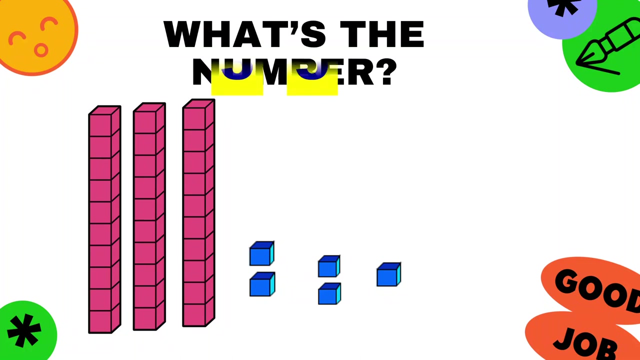 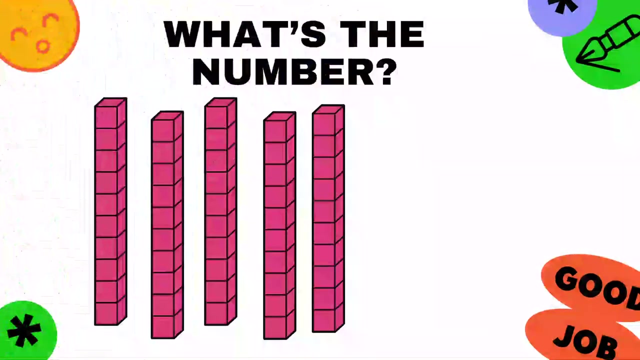 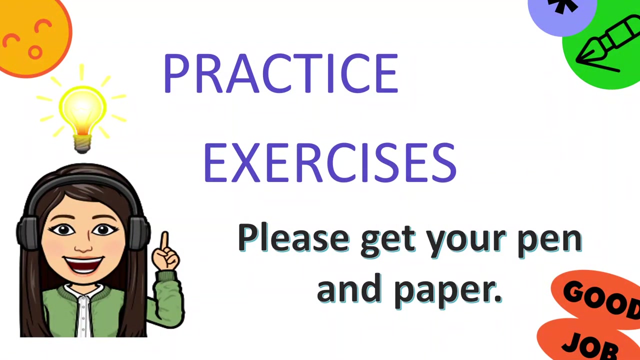 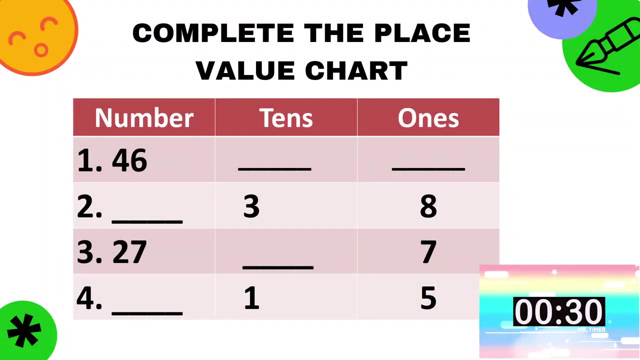